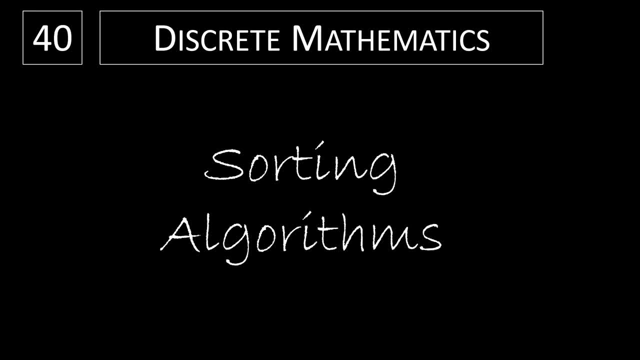 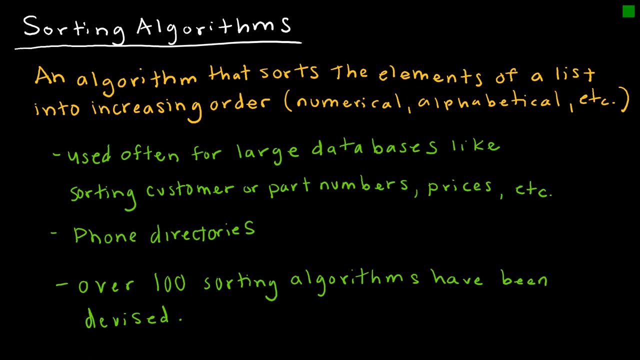 In this video, we're going to take a look at sorting algorithms. A sorting algorithm is an algorithm that essentially sorts the elements of a list into increasing order, and that is numerical, that is alphabetical. whatever it is that we're trying to order, that's how we would order them, So we often use sorting algorithms in large databases. 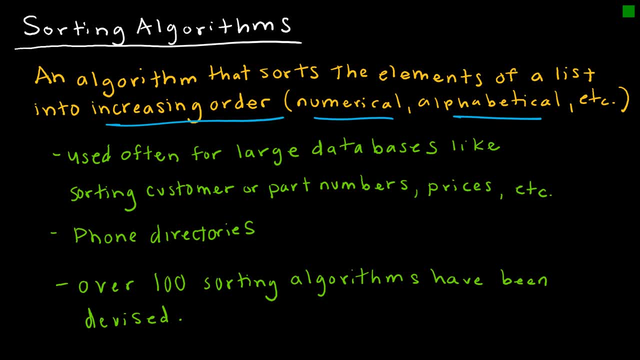 like sorting customer or part numbers, sorting prices, phone directories, obviously phone directories by last name, etc. There are over 100 sorting algorithms that exist out there in the world. We're not going to look at all 100 of them. you're welcome. So the first one we're going. 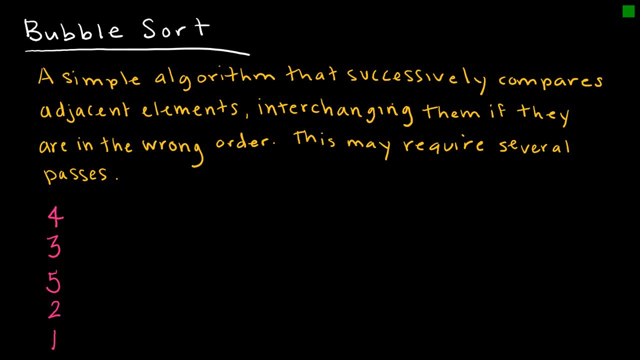 to look at is the bubble sort algorithm, and that algorithm basically compares adjacent elements, interchanging them if they're in the wrong order, and it may require several passes. So we're going to look at this one together, Pass 1,. I would look at 4 and 3, and my algorithm would say, hey, those are in the wrong number. 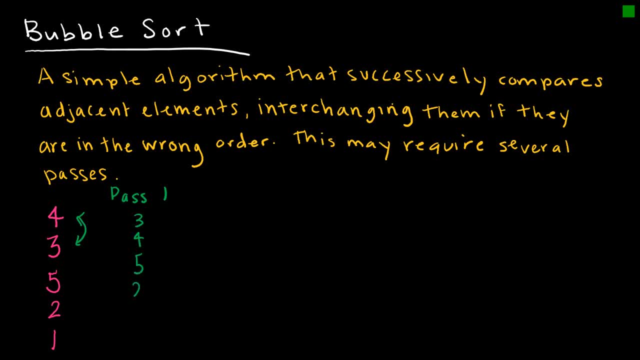 or the wrong order. so now I have 3,, 4, 5,, 2, 1.. Still in the first pass. I would then look at 4, 5, those are in the right order so I don't have to switch them. I would then look at 5, 2,. 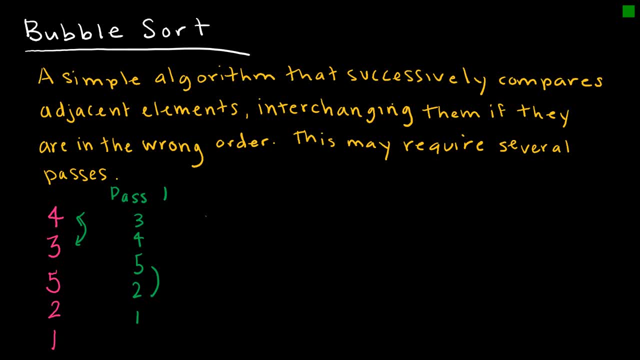 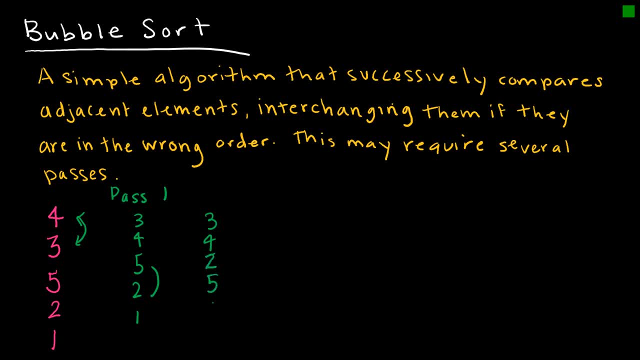 3,, 4, 2,, 5, 1, and then I would look at 5, 1, and 5, 1 is not in the right order, so I would have 3,, 4, 2, 1, 5.. That is all happening in pass 1, so I looked at each pair. Then in pass 2, I would 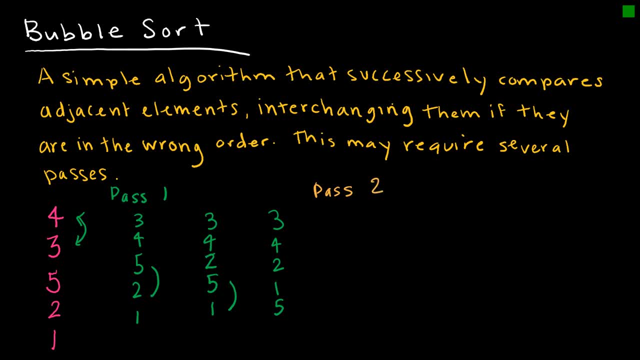 just then start at the top again. So pass 2,. I would say 3 and 4 are in the right order. 4 and 2 are not in the right order, so they're going to switch. so this is 3,, 2,, 4, and then I would look. 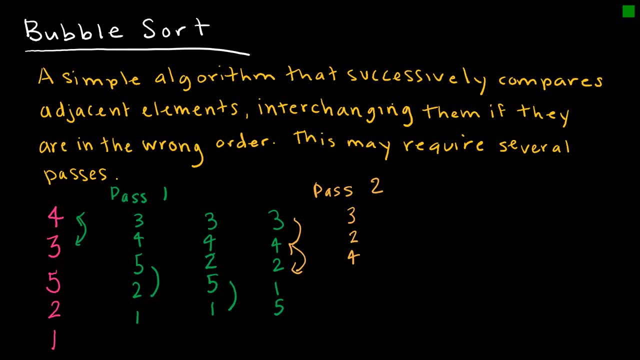 at 4, 1, because now it's a 4.. I'll go ahead and rewrite it like I did before. Then I'm going to look at 4, 1, those are not in the right order, which gives me 3, 2, 1,, 4, 5, and then I would 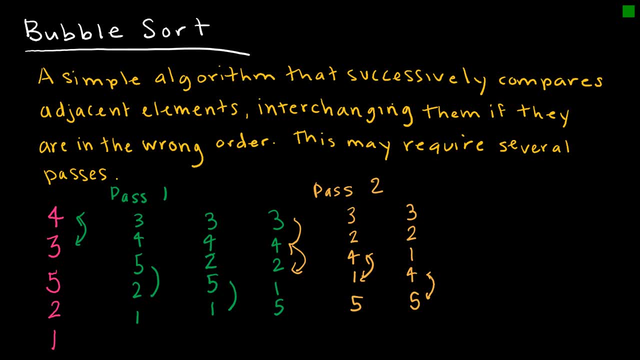 look at 4,, 5, and those are in the right order. So that brings us on to pass 3, where I start again at the top Pass 3,. I would look at 4,, 1, and those are in the right order. so that brings us on to. 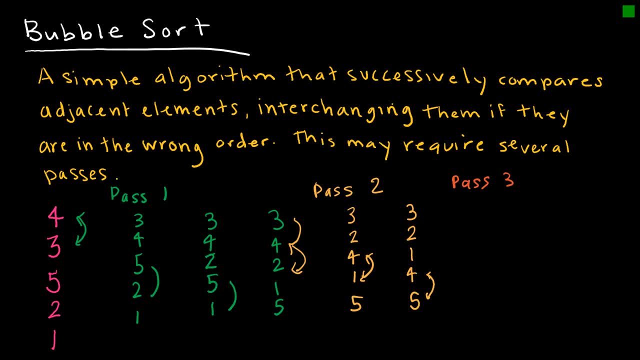 pass 4, where I start again at the top, And at the top I would say 3, 2 are not in the right order, so now it's 2, 3.. I would look at 3, 1, which are not in the right order, so that gives. 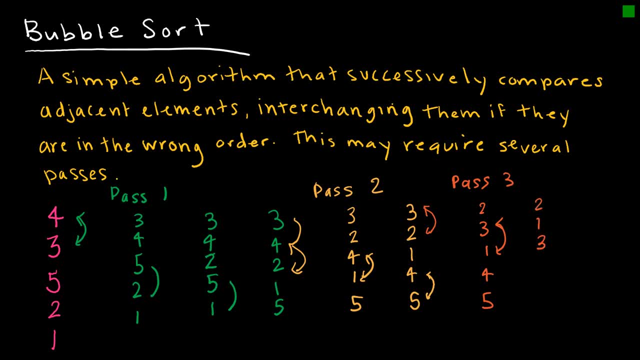 me 2, 1, 3.. Then I would look at 3, 4,, which are, and 4, 5,, which are. So now that brings me to pass 4,, where I would look at 2, 1, and say those are not in the right order. so that's now 1,. 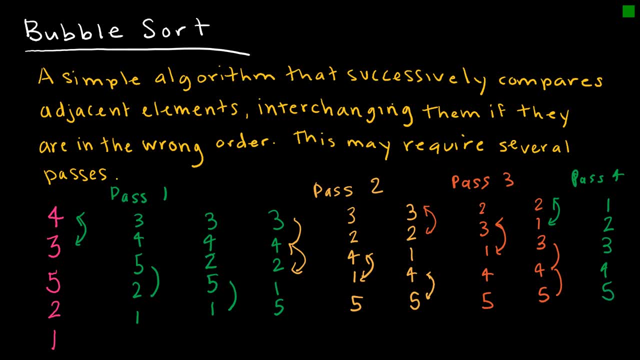 2. And then I would look at 2, 3, those are, 3, 4, those are, and 4, 5, those are. So it took me four passes to get where I wanted using the bubble sort algorithm. So, as you can see, 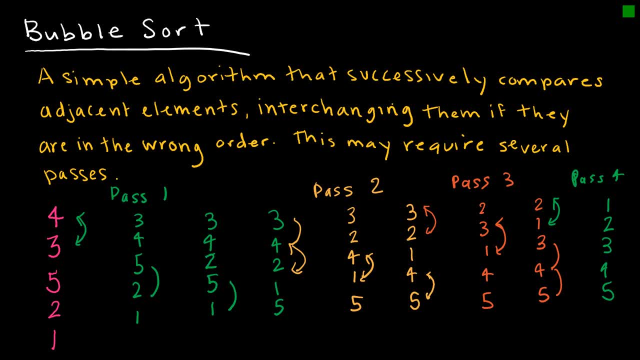 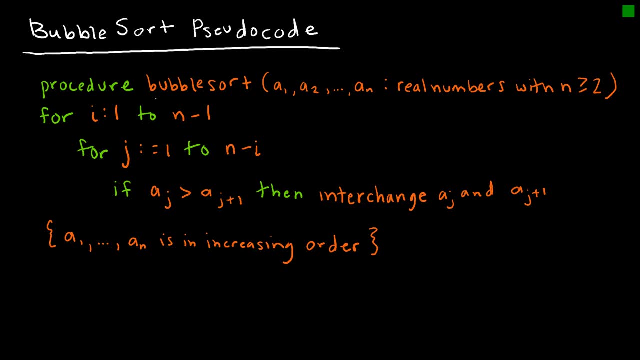 it's not necessarily efficient, but it is effective. So let's look at our pseudocode for our bubble sort procedure. We're looking at a procedure called bubble sort. We're dealing with a list of values with at least one val- or at least two. 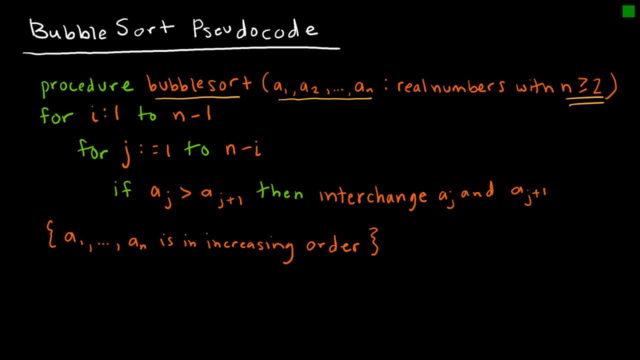 because if we had one value then we wouldn't need to sort them, we would just have one value. then we're saying: for I, which is of course the subscript I, from 1 to n minus 1, and then from J, which goes from 1 to n minus I, we're 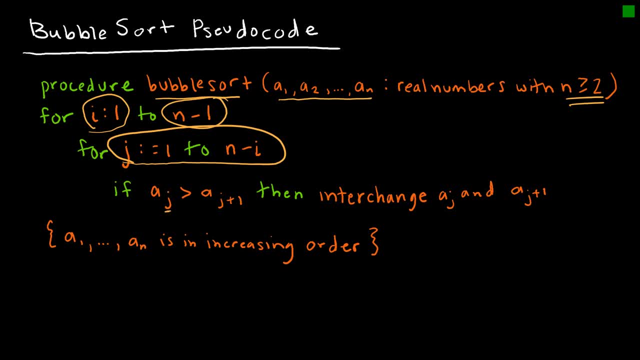 essentially saying: let's compare the two values, J and the value after that, and if the value is greater than the value that comes after that, then we have to interchange them and otherwise we don't, obviously. and so if we continue that procedure for all of those values, our output is that we get our values in. 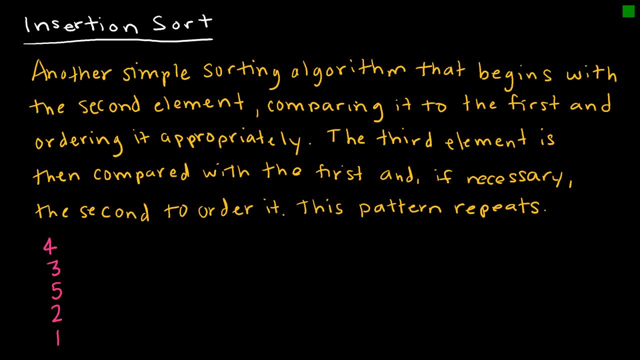 increasing order. the other sorting algorithm I want to talk to you about is the insertion sort algorithm, and the insertion sort algorithm essentially starts with our second value and says, hey, is this in the right spot? if not, let's put these two in the right spot. so, my first pass: I would end up with 3, 4 and then still have 5, 2, 1. my second pass. 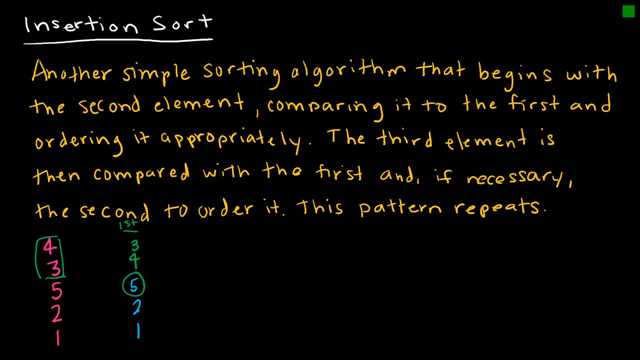 I would be looking at 5 and saying: is 5 in the right spot compared to 3, 4, 5? and so my second pass says: yeah, it sure is, but I still have 2, oops 2 and 1 to contend with. my third pass says: let's just look at the 2 where. 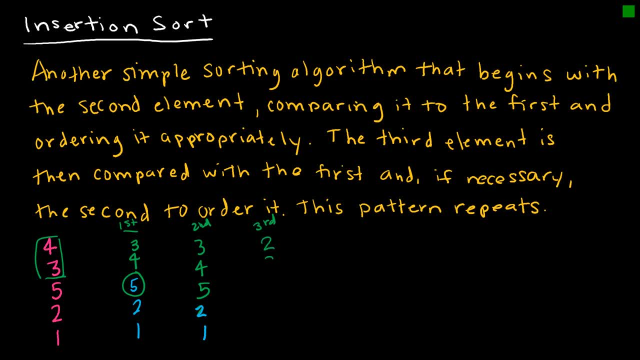 would the 2 go in that list and the 2 would go in front of the 3, 4, 5, which still leaves me with 1 to contend with, and then, in the fourth pass, I would be looking at putting the 1 where it goes, which is right at the beginning, and so 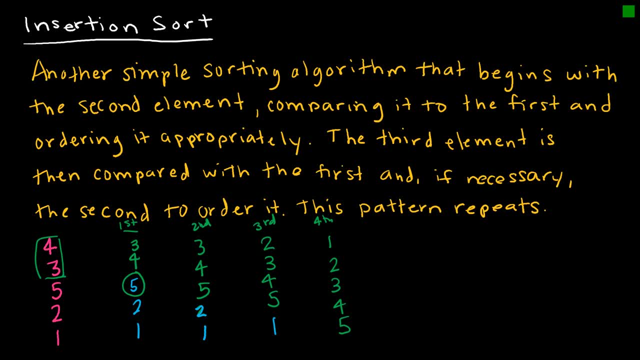 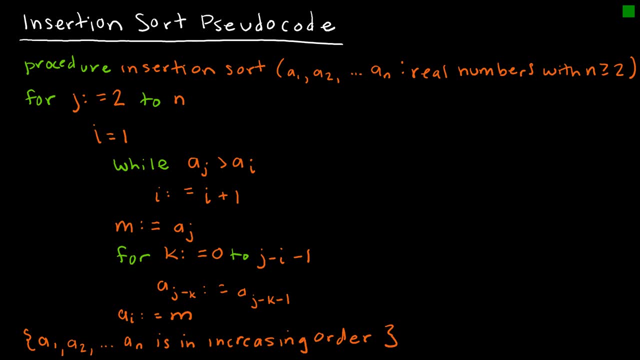 now I have everything in the proper order. so the insertion sort pseudocode has quite a bit going on, but essentially what it is saying is we have to take our values from 1 through n, with obviously two or more values, and we're saying, for J equals 2 to n, starting at I equals 1. 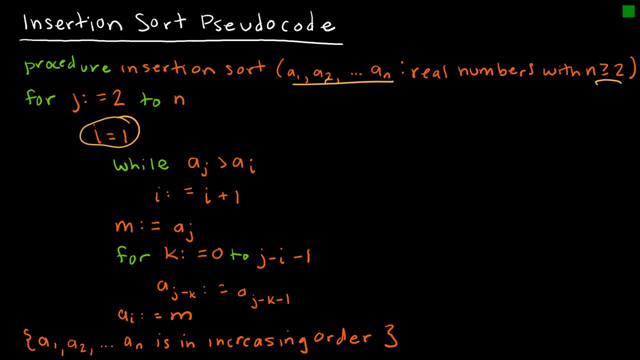 essentially, what we're saying is: let's compare 2 to 1 and switch their order if necessary. if not, then we go on to the next one and then essentially we're looking step by step for where does it go in the list that we have already essentially set. so that is the basis of the pseudocode for 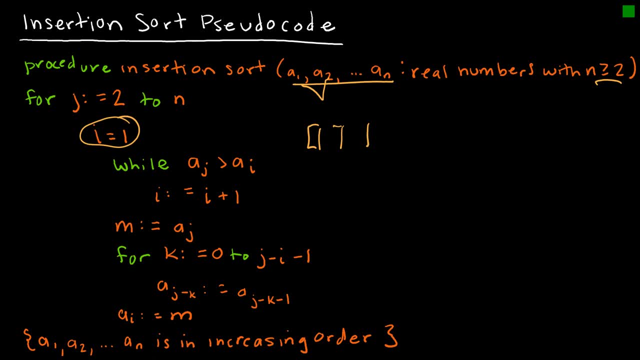 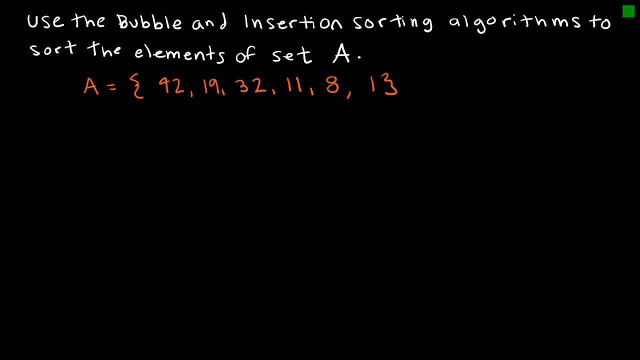 the insertion sort is that we're going to set those values and then our algorithm is going to check the locations to determine the correct placement and our output is going to be that our values are all in the increasing order. so let's take a look at a couple of practice and, again, keep in. 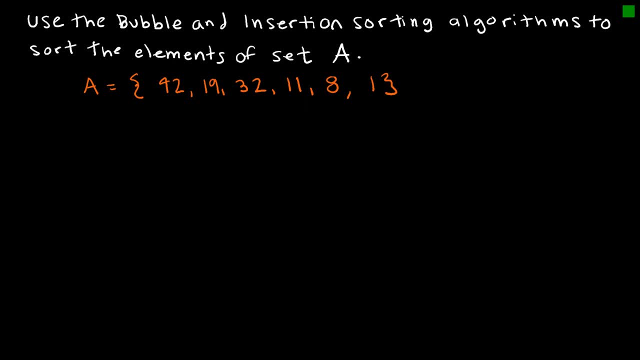 mind that we might have several passes through, but I'm going to start with the bubble sort, and what I'm trying to do is obviously sort these from least to greatest. so in my first pass I would compare 42 to 19, which would tell me that those two are not in the right order, and then I would 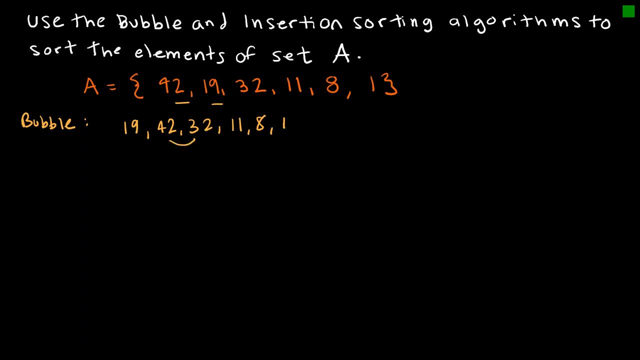 compare 42 to 32, which would tell me that those are not in the right order, and then I would compare 42 to 11, which tells me those are not in the right order. so 19, 32, 11, 42, 8, 1- remember, still on the first pass. I would then compare 42 to 8, and those are. 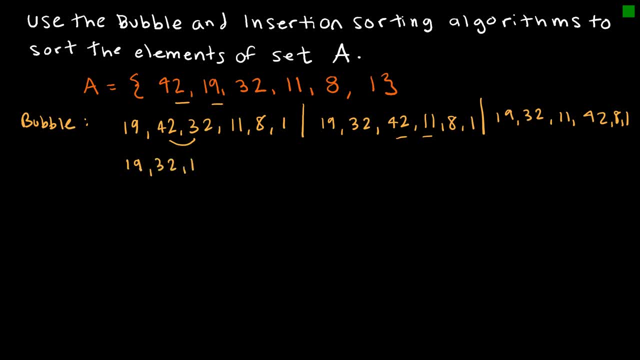 not in the right order. so 19, 32, 11, 8, 42, 1 and then 42 to 1. those are not in the right order. so 19, 32, 11, 8, 1, 42. that was all in the first pass. the second pass: I. 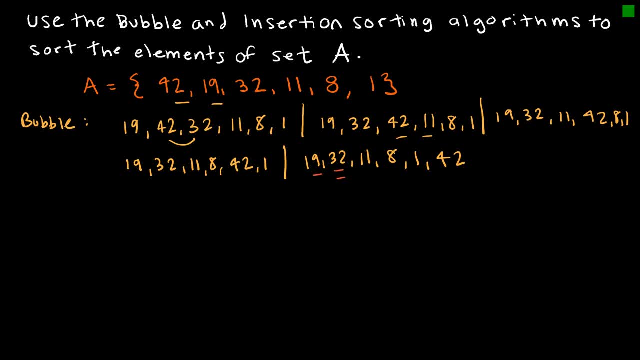 would compare 19 and 32. those are right in the right order: 32 to 22, quecheos between 19 and 32. I would compare 32 to 42, which gives me 19 and 32. I would compare you, t and make purchases or女, but a way based on the. 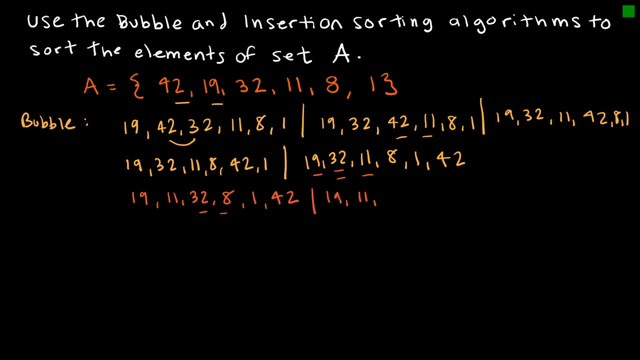 ui contes, cal 1999, contributed 12.11, which gives me 19, 11, 32, 8, 142. I would compare 32 to 8, giving me 19, 11, 8, 32, 142. I would then compare 32 to 1. so 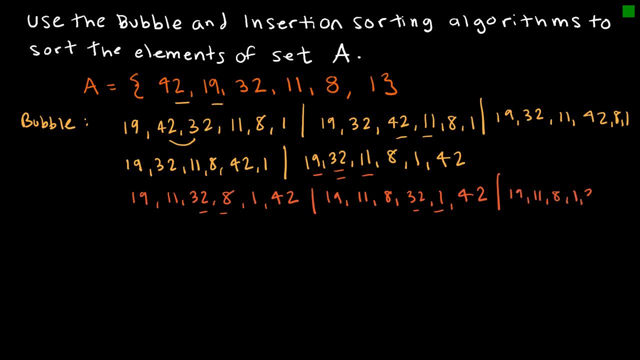 ayat kerroý one, so 19, eleven, 8, 132, 42 and lastly 2, 38, 12, joint, 21 and 7, 32 to 42, which is correct. So we're going to continue on to the next pass. 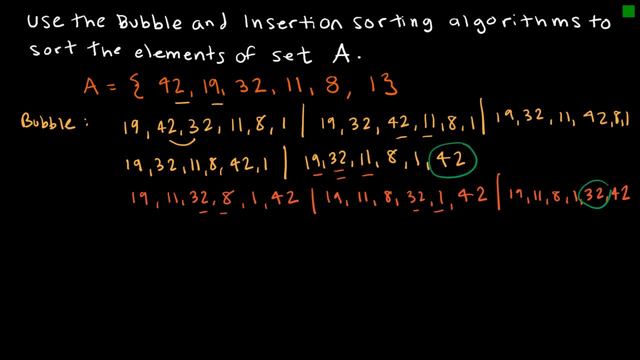 So notice, on my first pass, 42 is in the right spot and now 32 is in the right spot, And so now I'm going to start with 19 and 11.. Those are not in the right order. So 11, 19, 8, 1. 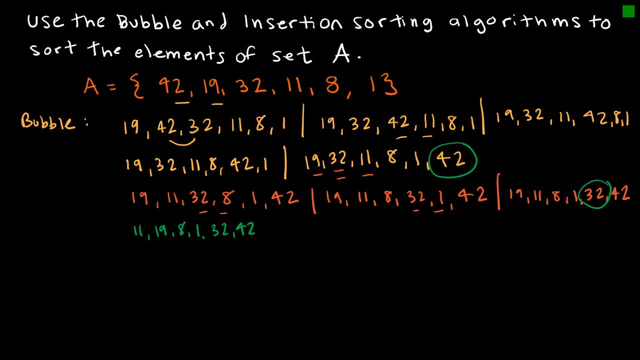 32, 42, and Then I'm going to compare 19 and 8. so I've got 11, 8, 19, 32, 42, and Then I'm going to compare 19 and 1. so 11, 8, 1, 19. 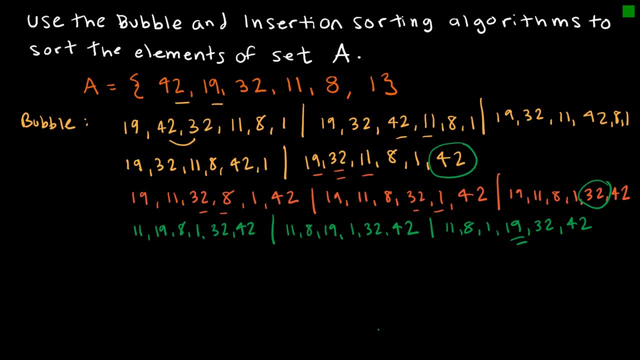 32, 42 and again. I now have another one in the correct order, Because the rest of them are okay. Now I'm going to go to my next pass. I'm going to compare 11 and 8, so I get 8, 11, 1. 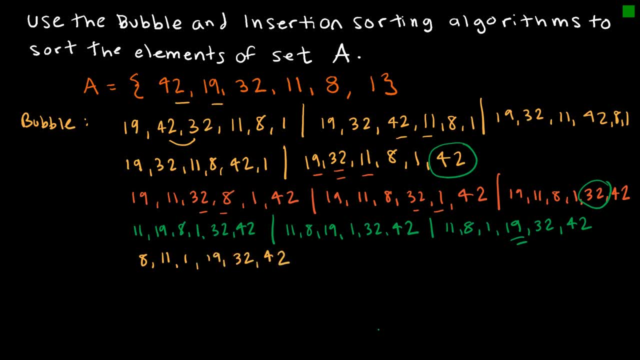 19, 32, 42. Compare 11 and 1, Giving me 8, 1, 11, 19, 32, 42. that passes over and I now have 11 in the correct spot. and then in my last one, I'm going to get 1- 8 by comparing the first two terms. 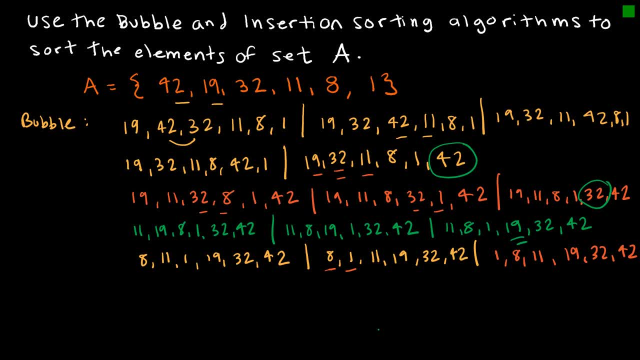 19, 32, 42. So now I have used the bubble sort and my elements are sorted correctly. Hopefully I can fit in the insertion sort correctly. So let's look at what that looks like. My insertion sort starts with the first two and places them in the correct order. 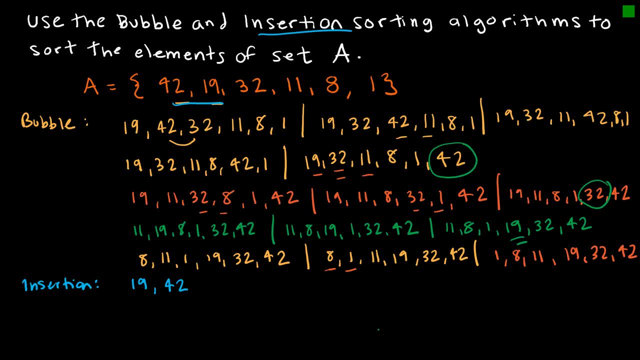 so 1942. the rest of them are still to be placed. My next pass would then compare this 32 and Basically compare it against to both the 19 and the 42, And so it would place correctly the 32 between the 19 and the 42. 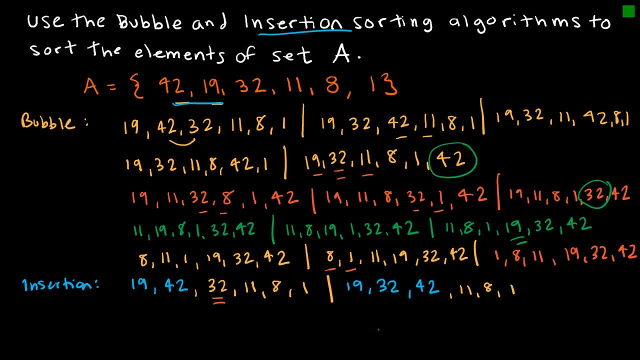 But still leave 11, 8 and 1 to be placed. My next pass would put the 11 in the proper spot, So I would have 11, 19, 32, 42. keep in mind that process is involved because it's actually comparing it.